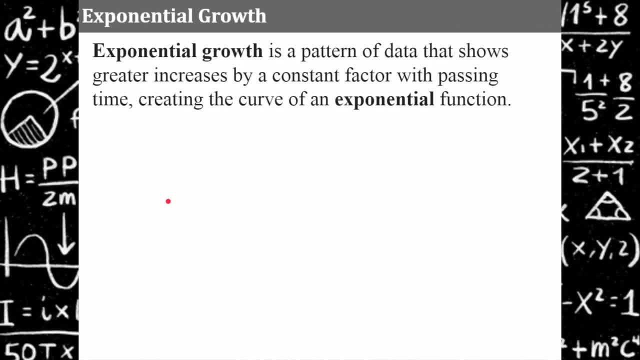 Let's start with exponential growth. Exponential growth is a pattern of data that shows greater increases by a constant factor with passing time. This creates the curve of the exponential function. So in a previous lesson we talked about exponential functions and how to graph them. Now we're going to talk about specific examples of real-world problems. 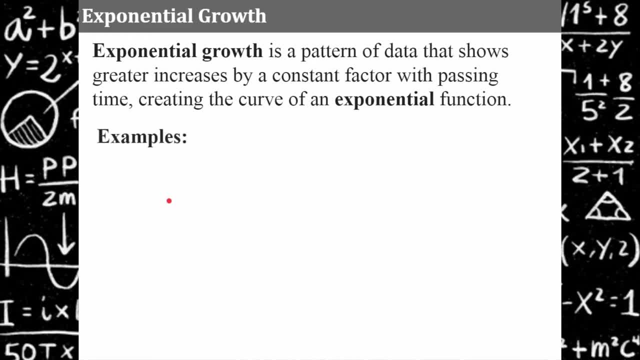 that show growth. Here are some real-world examples: Food spoiling: Mold growing on spoiling food is an example of exponential growth. Pandemics: COVID-19 is an exponential function Compound interest, So the interest you earn in a savings account every. 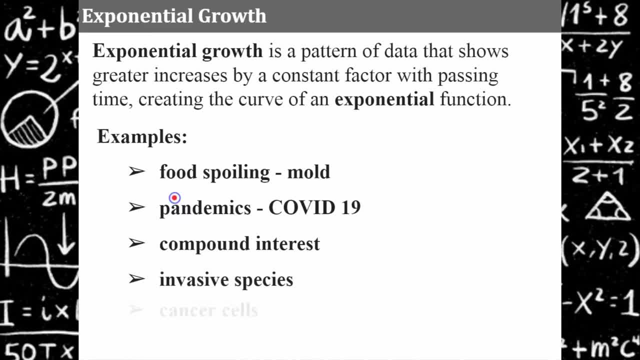 month, An invasive species, Cancer cells, Fire. So fire grows exponentially. So what happens here is things are multiplying, They're growing by a factor. So when you start with one person infected, that person infects with a virus. They could infect many people and then those many people. 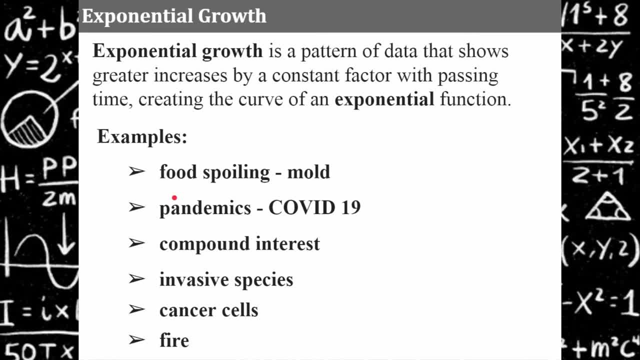 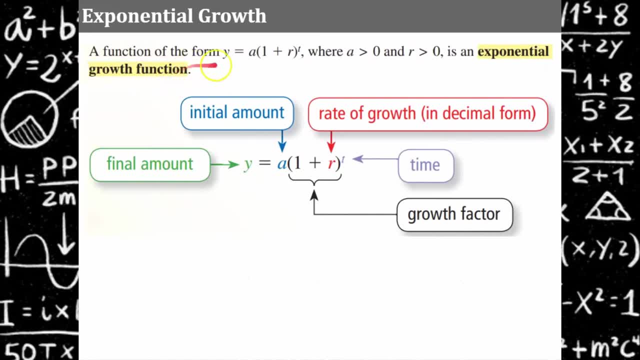 go on to infect many more people, So it just kind of spider webs out, and that's what we call an exponential growth function. An exponential growth function is written in this form: Our base is one plus a rate of growth. Okay, so sometimes this rate of growth is called is. 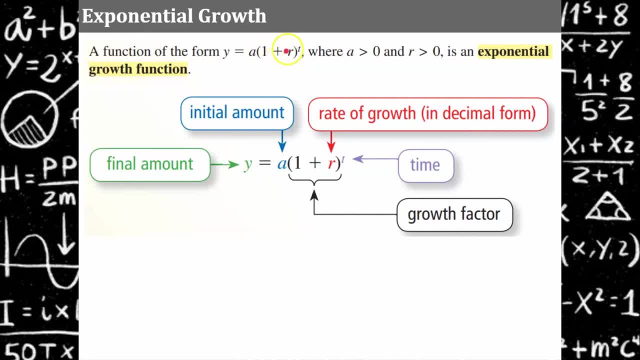 referred to as a percent and you're going to write it as a decimal and you'll see a decimal in here, But you have the one whole. So when something's growing, you have what it was and it keeps growing. So let's talk about money. 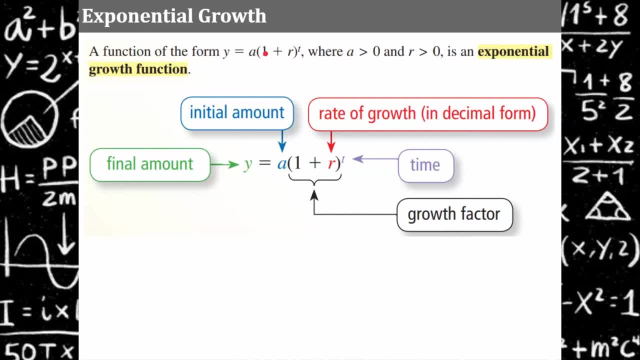 The next thing you want to look at is interest. There's a good business model for putting it into your savings account. So living your life. if you take your income for a minute, if you put $100 dollars in your savings account and you do not touch it- meaning you don't withdraw and spend it. 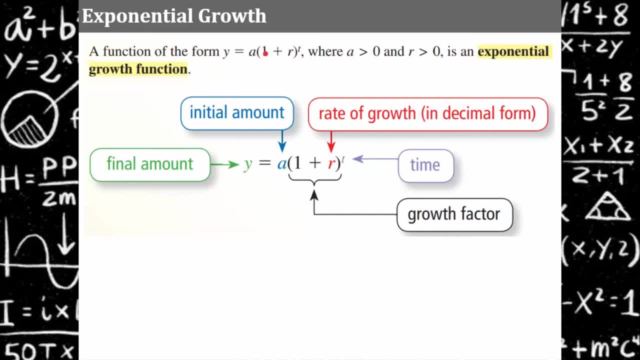 you're going to get interest on that in one month. So you're going to have $100 of the money you had plus the percent of interest added into the account. The next month you're going to have on the interest that you've earned in the previous month. 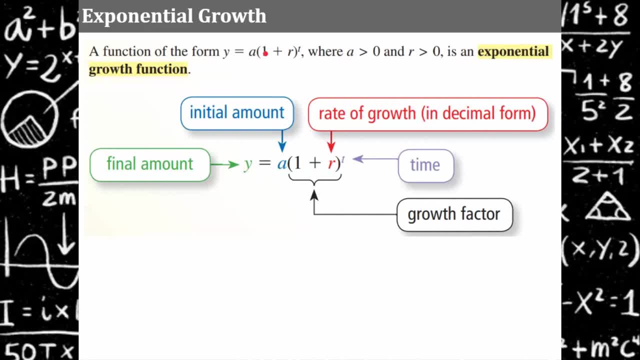 So you can see how we call that compounded interest. So this A is your initial amount. So if we were going to invest $100, we would say $100. And that one represents that 100% of that $100. So you're always going to have that if you don't touch it. 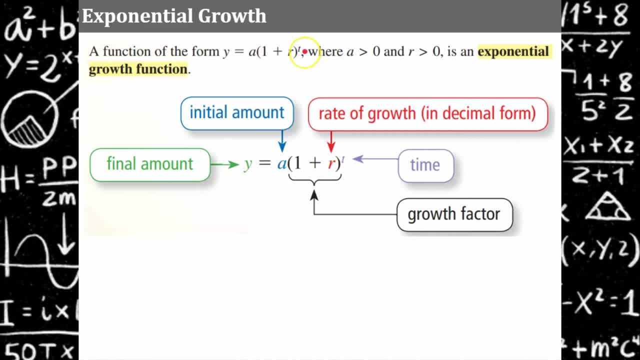 And then it's going to keep compounding And this exponent would be the number of months that you keep it in the bank. So it could work a different way. You know, initially there were three cancer cells in a body And those don't go away. 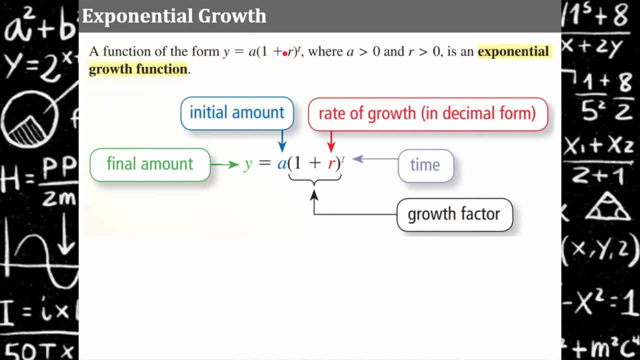 Those continue, each of them continue to grow and spread more cells. So A is always going to be greater than zero, because then you wouldn't have a function, because zero multiplied by anything is zero. And R must also be greater than zero because otherwise it wouldn't be increasing. 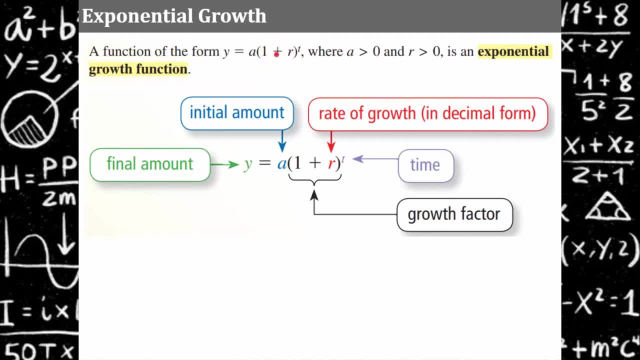 Your base would be one And you know from an exponential function, the base must be greater than one. So right here we have our initial amount. This is our final amount after the period of time. So the rate of growth. So whether you're talking about a flu, mold or interest in a bank, it's growing over time. 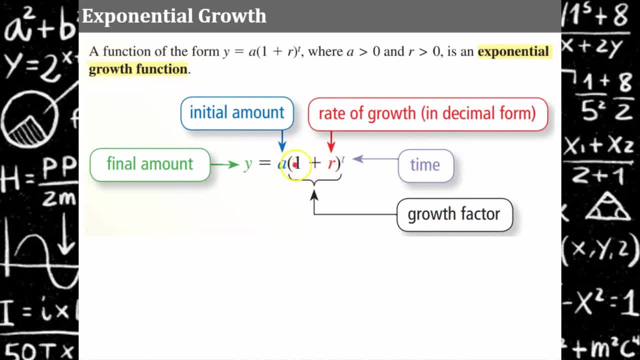 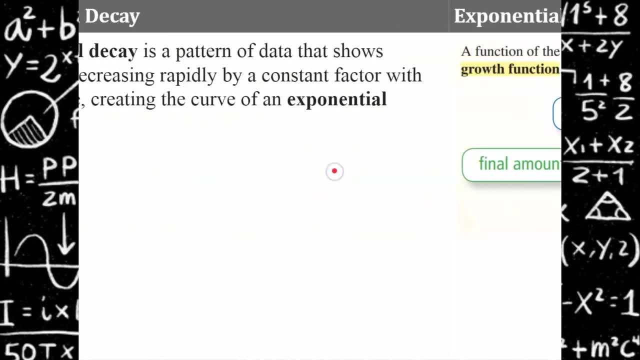 And this is our growth factor, Remembering that one is there to represent 100% of what you already have, plus a new rate. Exponential Exponential. Exponential Exponential decay is a pattern of data that shows something decreasing rapidly by a constant. 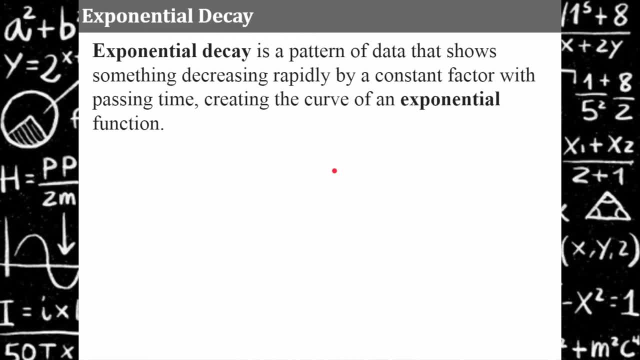 factor with passing time, creating the curve of an exponential function. So examples of exponential decay are value of a car. That doesn't decrease at a constant rate. So when you drive a car off a lot, brand new or not, it starts decreasing in value. 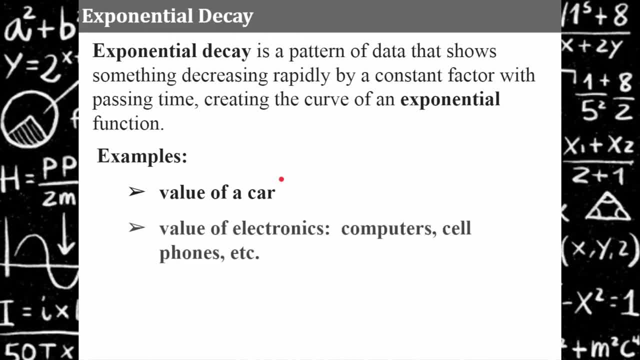 And it's not at a constant rate. It's an exponential function. Values of electronics are a perfect example: Computers, Cell phones. I'm sure you know that as soon as you have one in your possession, it's no longer worth what you paid for. 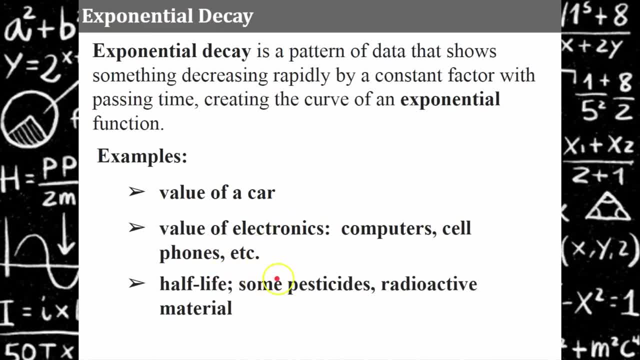 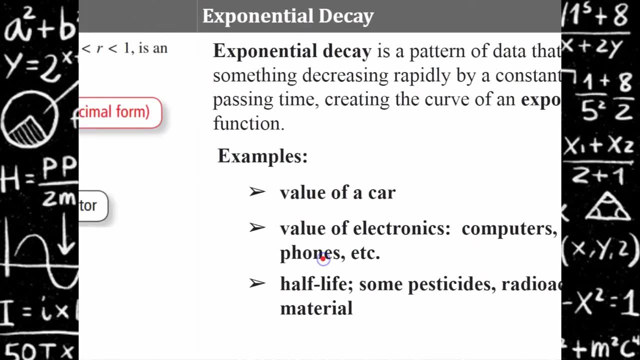 And then sometimes you refer to half-life. That's a science term. We talk about that as far as pesticides disintegrating into the ground and how far it takes to eradicate itself. Radioactive material is another one, So you'll hear about those later on in science courses. 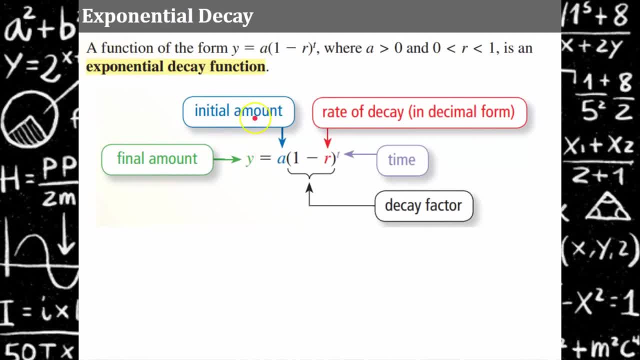 Let's talk about what the exponential decay function looks like. Let's talk about what the exponential decay function looks like when written as an equation. So we have our final amount here. That's what it's equal to. You still have an initial amount. 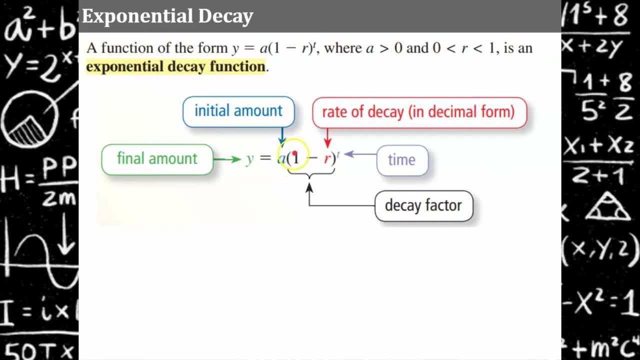 You started with something. So let's say that you've bought a car. Maybe your car costs $30,000.. That's your initial amount. So you have your factor of one here. You have that one showing that we have a decay factor. 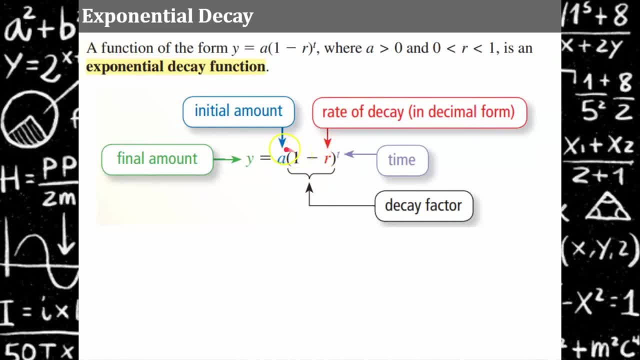 So the rate of decay is subtracted from that, because we're going to decrease our initial amount- Okay, Some cars gain value but some cars do not. And then your exponent is going to be the amount of time. So you could calculate if you knew the rate of decay or the rate of decrease of the value. 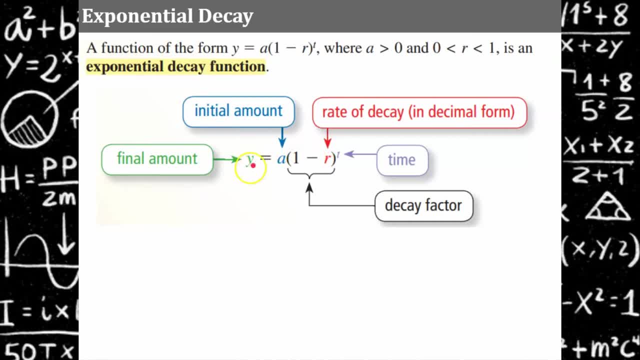 of a car or a cell phone, you could project what it would be worth. One fun fact to know is we've learned in a previous lesson that an exponential function is never equal to zero. It never crosses the x-axis. So I always like to ask students in my class every year a question about the value of a. 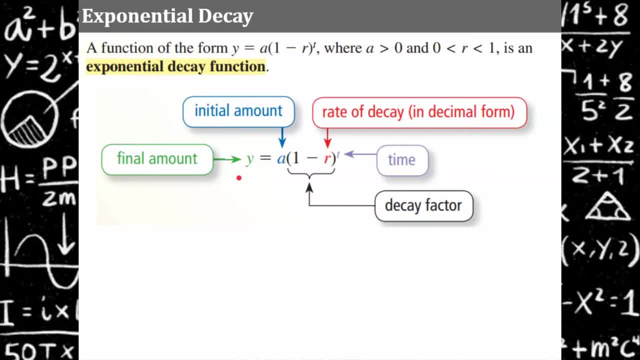 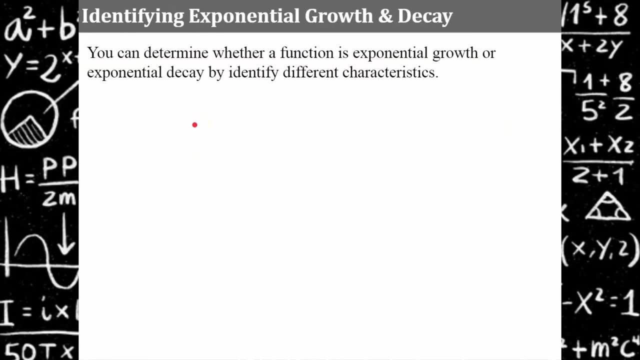 car And they answer: you know a hundred years and it will never equal zero. So think about it. You always even just have scrap metal. Okay, But an exponential function will never equal zero. All right, Let's talk about identifying an exponential growth and decay function. 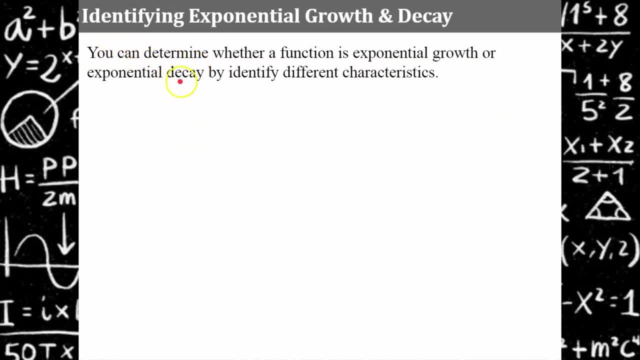 So you can determine whether a function is exponential or growth or exponential decay by identifying different characteristics. So for exponential growth, if you're going to look at an equation, the value of the base, the power, is going to be greater than one. So if you are asked that you look at the base of the 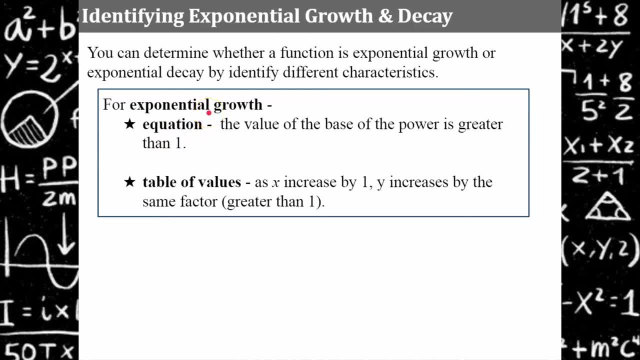 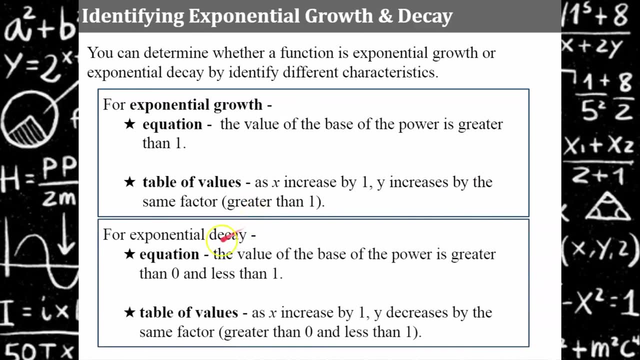 power. If it's greater than one, you know it's exponential growth. If you're looking at a table of values, you always have to see x increasing by one as y increases by the same factor that's greater than one For exponential decay. in an equation, the value of the base of the power is: 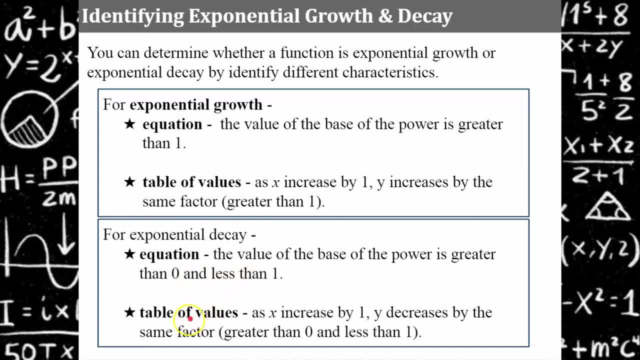 greater than zero and less than one. Table of values. as x is increasing by one, y is decreasing by the same factor. It has to be greater than zero and less than one. So let's go ahead and see if we can identify these characteristics in a few examples. 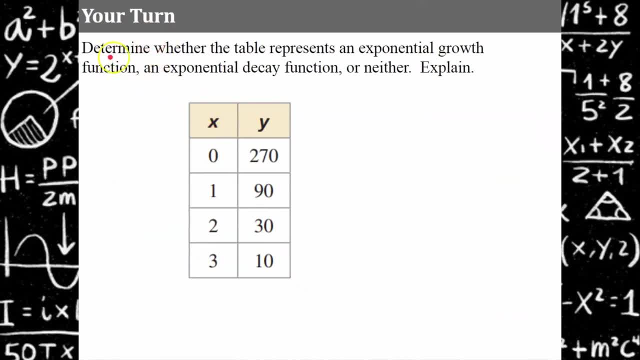 So I say: your turn here, but I'll model this one for you. So we want to determine whether this table represents an exponential growth function or an exponential growth function, exponential decay function or neither, And we want you to explain. So first I'm going to identify. 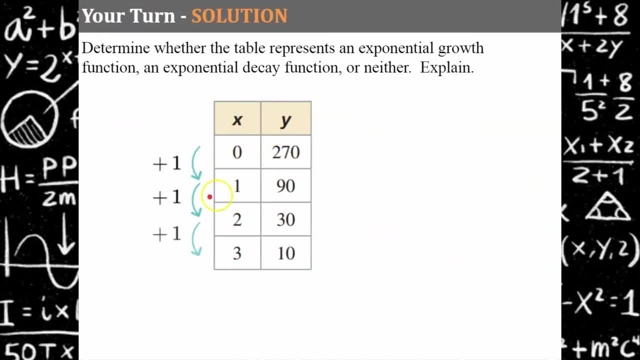 that the x is increasing by one and the y values are decreasing by a factor of one-third. So 270 times one-third is 90.. 90 times one-third is 30.. And 30 times one-third is 10.. So, because this is, 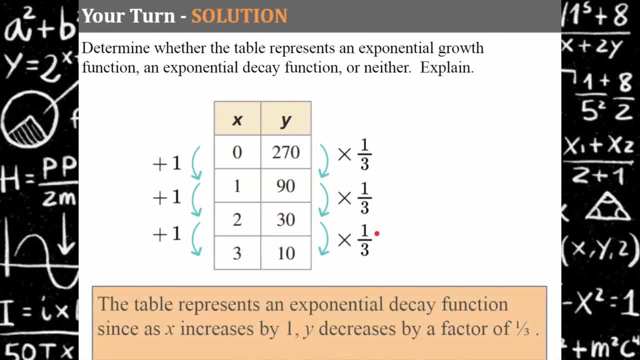 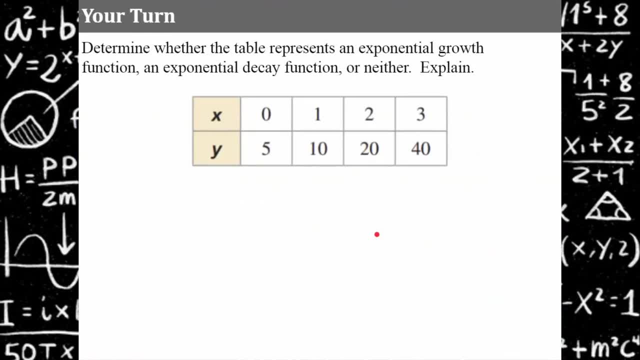 decreasing by a constant factor of one-third. we know that this table is going to be greater than zero, So this table represents an exponential decay function. Okay, your turn. I would like you to pause this video. go ahead and determine what kind of function this is: either growth or decay. 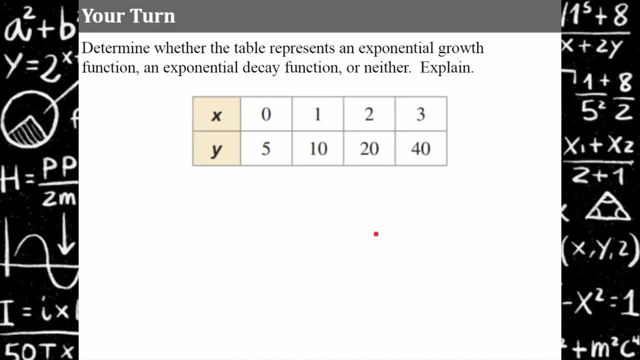 or neither, and be able to explain. Come back and hit play when you're ready to check your work. Welcome back, Let's see how you did So. the x is increasing by one. the y values are increasing by a factor of two. 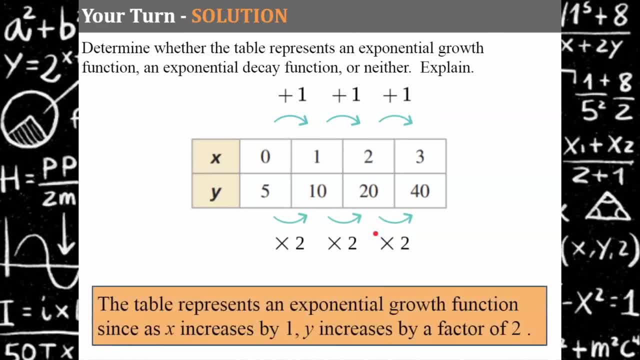 So this table represents an exponential growth function. six is since: as x is increasing by one, x is increasing by one, y increases by a factor of two, richest increase. Try this one. Please pause, Come back and hit play when you're ready. 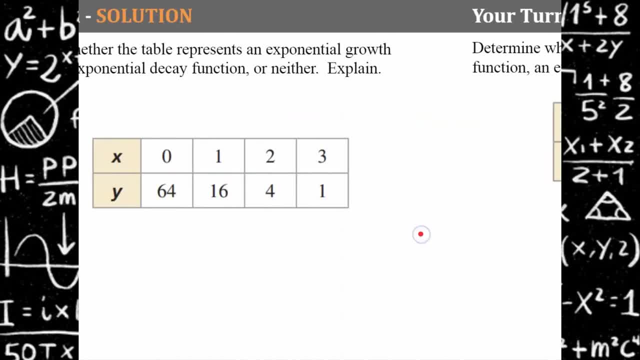 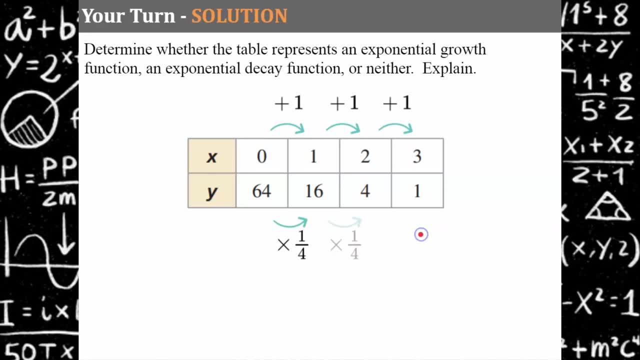 and hit play when you're ready. welcome back. let's see how you did So. as x increases by one, y decreases by a factor one-fourth. Therefore, this table represents an exponential growth function. So This table represents an exponential decay function, since, as x is increasing by 1, y decreases by a factor of 1- 4th, 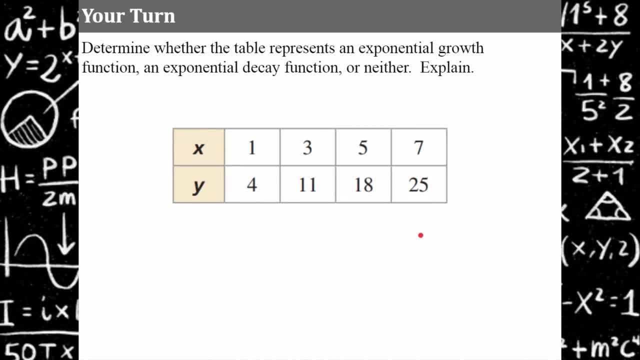 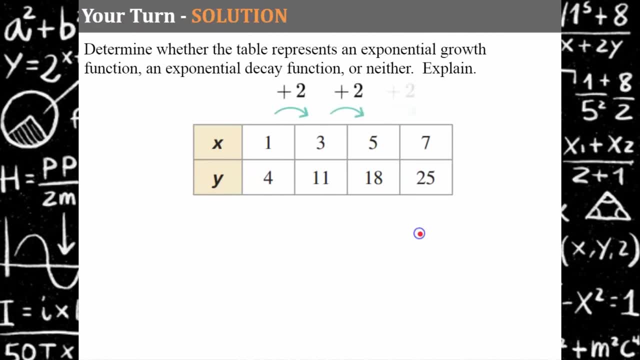 Here's another one for you. Please pause and come back and hit play when you're ready. Welcome back. Let's see how you did, As x is increasing by 2, y is increasing by 7.. So this table represents neither. 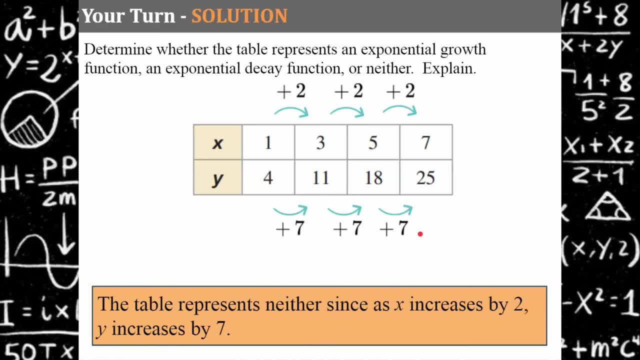 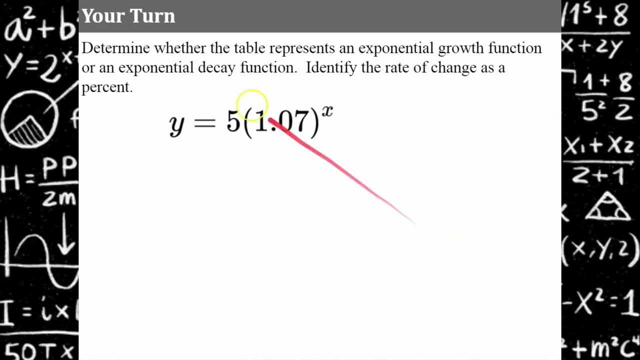 This is actually a linear function because, as x is increasing by 2, y is increasing by a constant rate of 7.. So it's not increasing by a factor, but a constant rate. Now we have an equation. I'm going to model this one for you, even though I say: your turn. 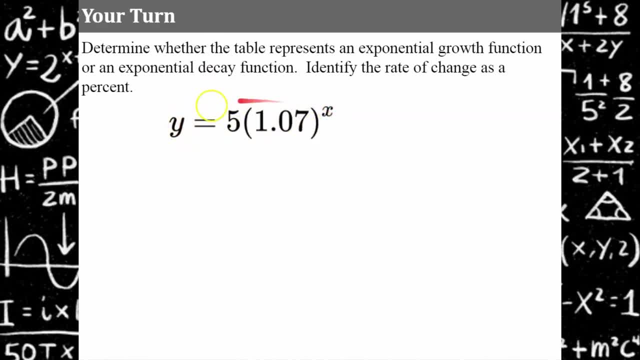 We want to determine whether or not this represents an exponential growth or decay function and identify the rate of change as a percent. So here we go, The base of the power. so here's our power. the base of the power is greater than 1.. 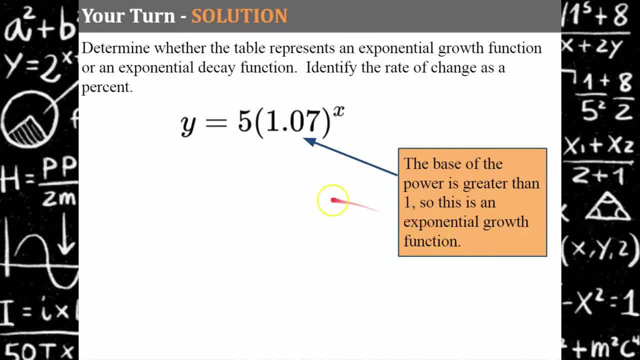 So I know that this is an exponential growth function. Now I want to identify the rate of change. So remember, an exponential growth is a hundred percent of the initial amount plus the rate of change. So here we have a rate of change that is 7 percent, because 0.07 is. 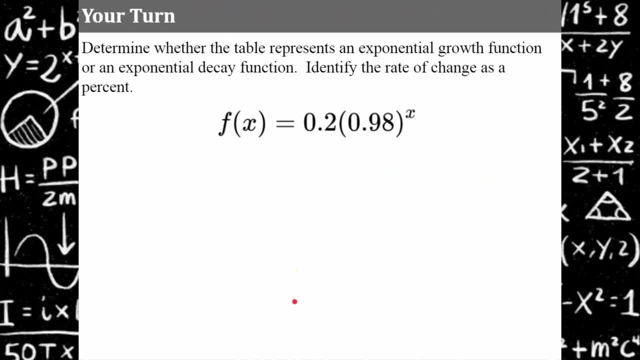 7 percent. Okay, your turn. Please identify whether or not this is exponential growth or decay and identify the rate of change as a percent. Please pause, come back and hit play when you're ready. Welcome back, Let's see how you did. 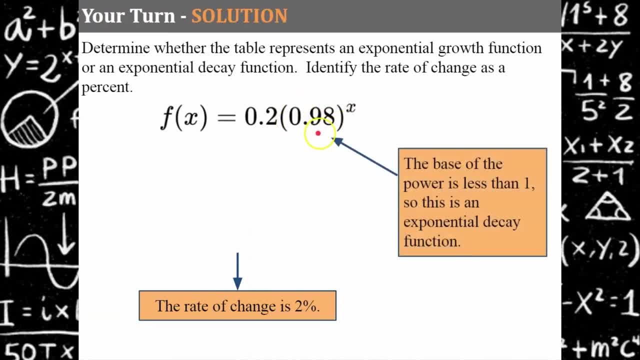 So we have a base of less than 1, so this is an exponential decay function. and the base of this power is less than 1, so this is an exponential growth function. And remember, we're going to subtract that, We're subtracting from the whole, so our one whole. 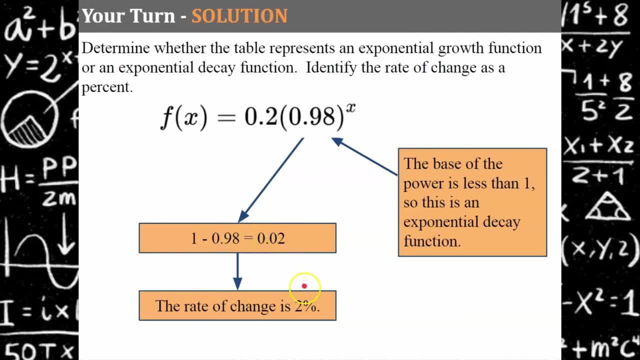 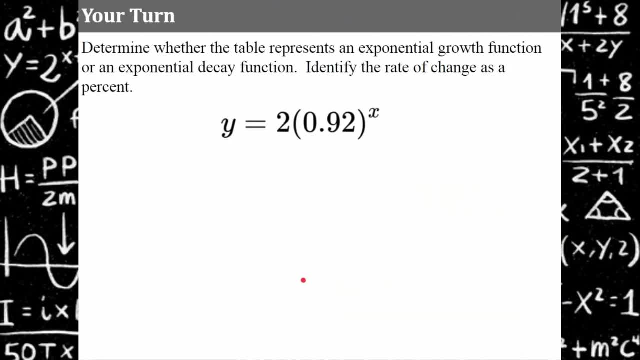 subtract the 0.98 gives us a rate of change of 2 percent. Here's another one for you to try. Go ahead and pause, come back and hit play when you're ready. Welcome back, Let's see how you did. 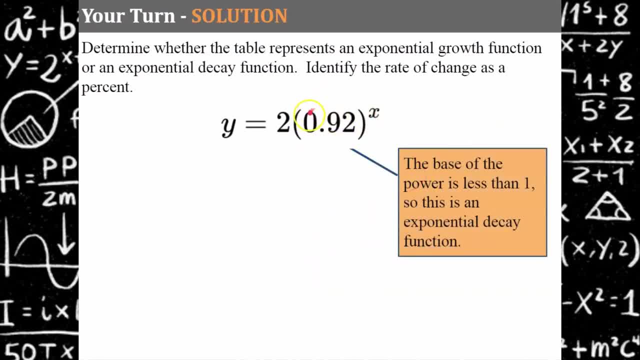 So the base of this power is less than 1, so this is an exponential growth function. Remember, we're adding to the 100 percent, so we're subtracting from the whole. so this is an exponential decay function. We're going to subtract the factor.